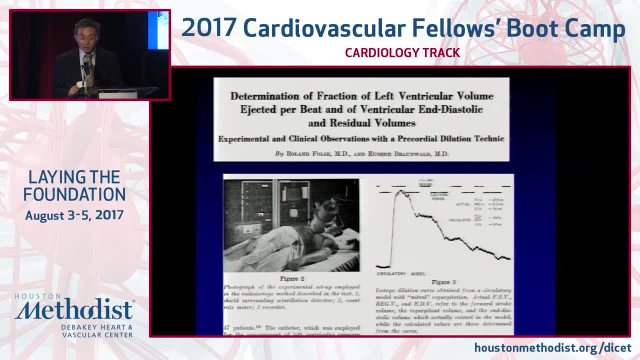 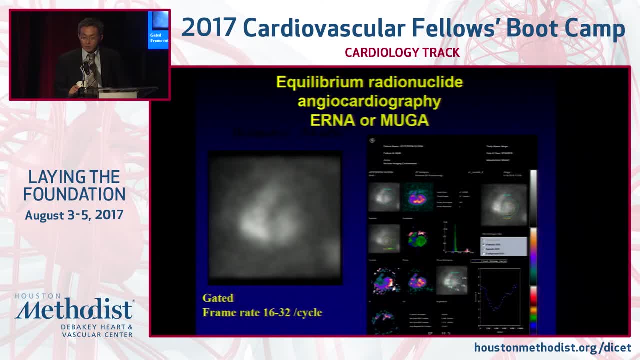 started with assessment of ejection fraction. This is a paper by Dr Jim Brownwall when he was in NIH, So just to give you a perspective, And this is a MAGA. In the old days it used to be a gold standard for EF assessment. Now they will still use it in rare occasion because 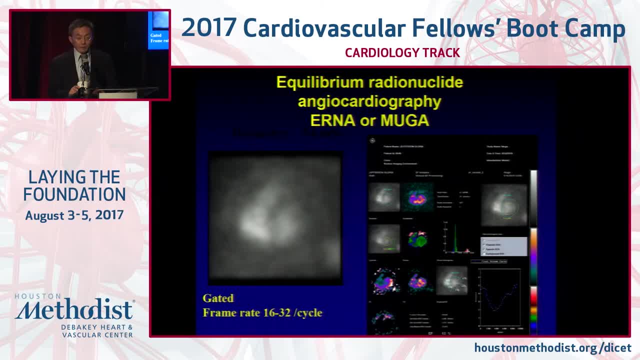 we have so many other tools to assess LVEF, But inpatient, for instance, cannot go to MRI. had a very poor cardiac window For ultrasound. this will be a very good substitute. I'm sorry the movie is not playing Okay, so stress. myocardial production imaging. 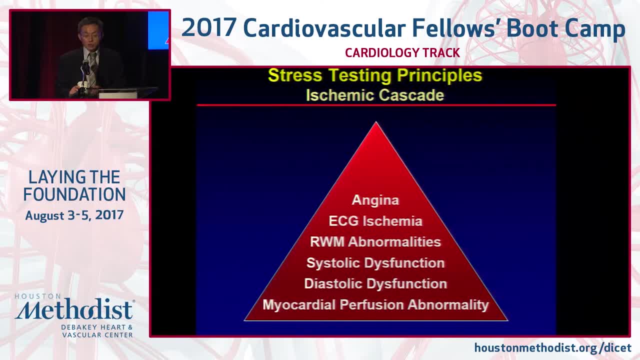 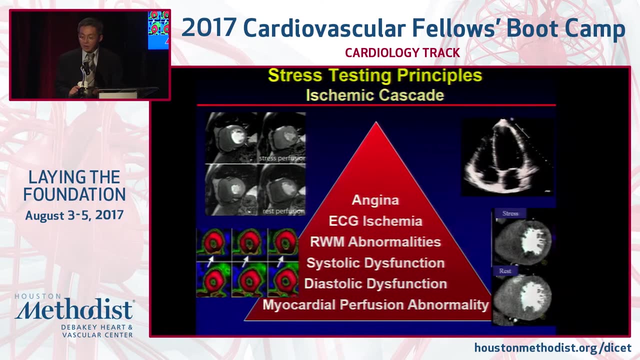 You know the rationale behind doing production imaging. stress is- it's called stress test- ischemic cascade. So in the absence decrease of blood flow, first you get a profusion abnormality, then you get systolic dysfunction, wall motion abnormality and ECG changes and then you 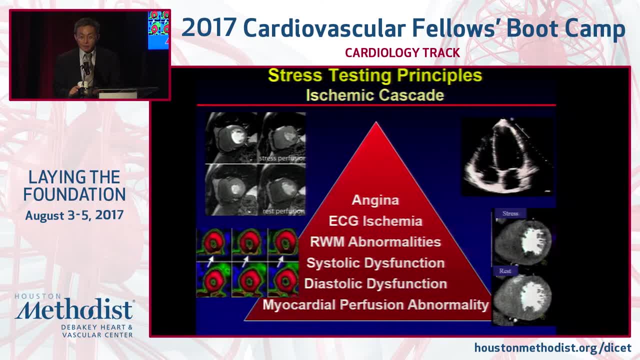 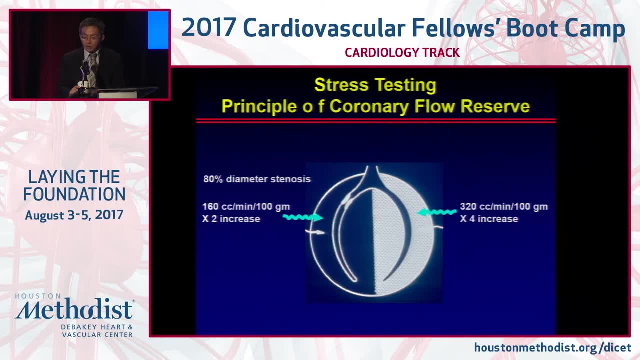 have symptom. So myocardial profusion abnormality is one of the first sign of ischemia. Okay, And this is based on this principle that we have differential coronary flow reserve in the presence of significant stenosis, You get more uptake in ischemia. okay, 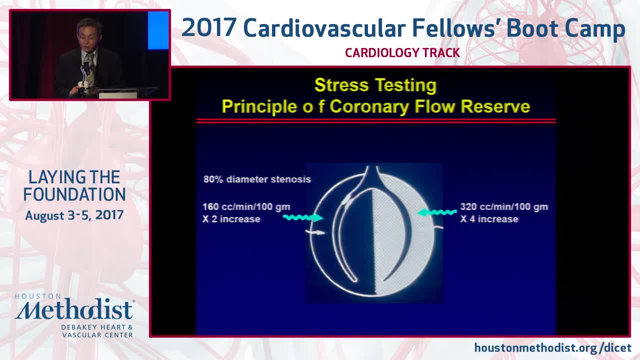 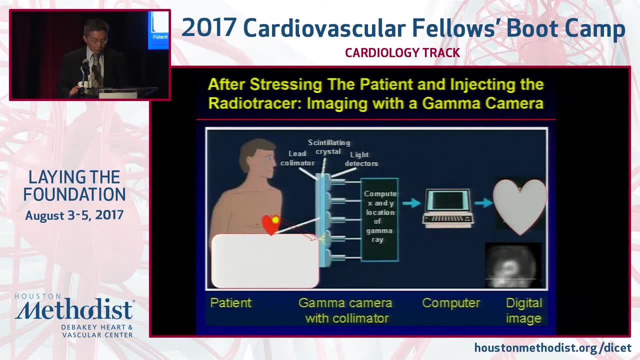 So the first sign of ischemia is coronary bed with no obstruction, compared to the one with obstruction, okay. And how we do it in the nuclear medicine. So we nuclear cardiology, we inject radio tracer who goes to the heart, get uptake by the heart and then we put the 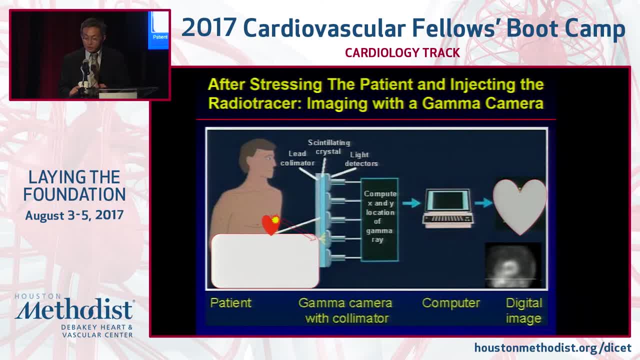 camera around the patient, The photon leave, the heart is captured by the crystal and then, through some sophisticated computer algorithm, you recreate the heart And then with the spec we slice this in different axes. Okay, To give you a 3D representation of the heart so we can localize the defect. And there's. 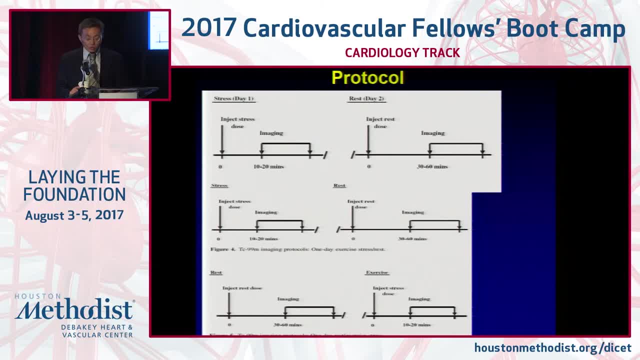 several protocols. The original protocol the most. the gold standard is do the stress portion and rest portion in two different days with two different injections. But because it's a little bit cumbersome for a patient to come back in two days, protocol was modified. 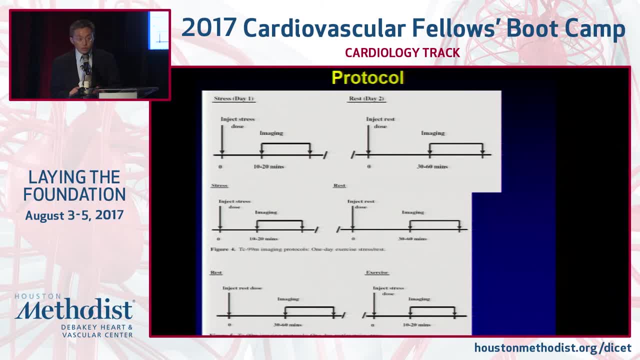 to fit into one day. You can do rest first or stress later, or stress first or rest later. The method is we prefer to do stress first, especially in a patient without history of coronary disease, because if you have a normal stress you can stop there. 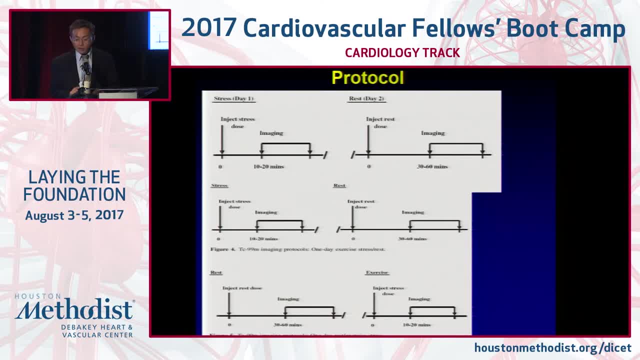 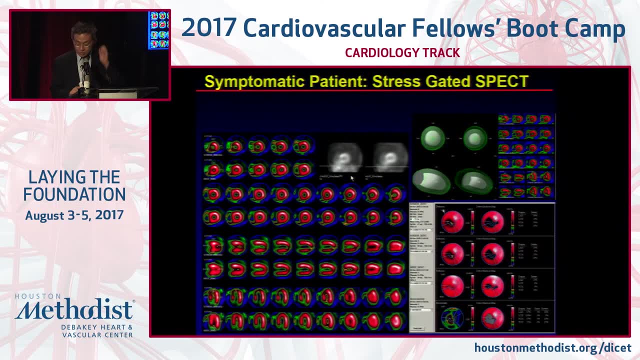 Okay, So you can imagine much more convenient in patient receive much less dosage. This is an example of a patient with symptom. you can see there- The top part is the stress images and the bottom part is the resting imaging. You can see a clear defect in anteroceptal. 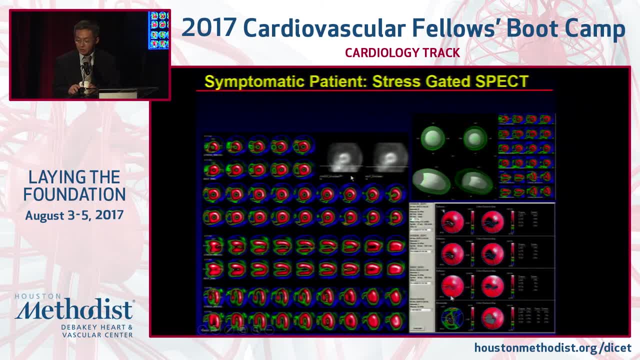 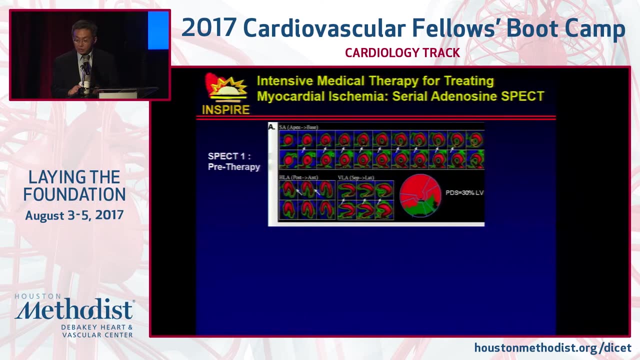 wall And here in Methodist, Methodist will do routine quantification, which is very important for follow-up and to see the therapeutic impact of the defect size. Okay So, and the other important use for this technology, especially quantification, as I mentioned. 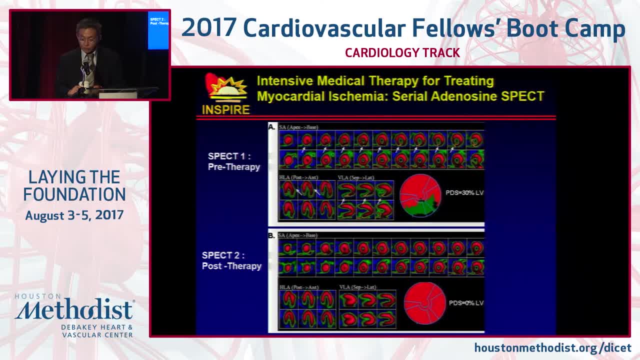 earlier. this is a patient with non-ST elevation. MI had an inferior wall defect with quantifications, as I said earlier, but the condition is quite similar to that of the patient. This doesn't require any much depth, but it does require some time to develop the Fox luster bypass. 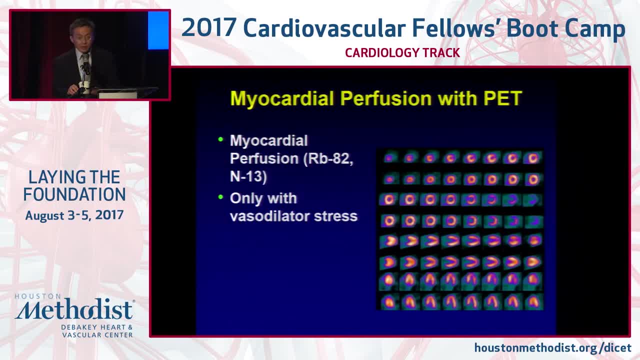 method. Now let's talk about PT, Let's talk about the CT. the CT is a very… It's a very… It's an ascending path which has very low level of dih eradication effect, as you can see. 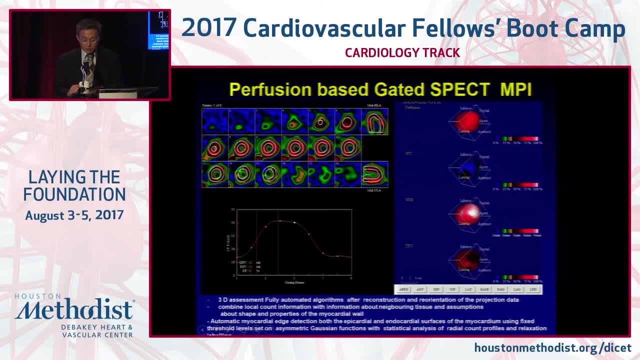 It's very high level of dih eradication. It's going to be the same with PET, It's going to be the same with CT and we're going to think about accelerated EMT, but that's going to be a different thing. 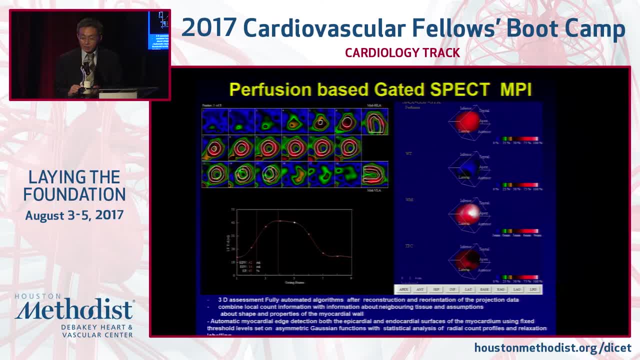 tracer could be done in conjunction with exercise. The other advantage- I would say bonus- of doing a micro revolution imaging is you don't only you're not only getting the profusion information, you're also getting the functional information in terms of LV size, LVEF, which also very important in addition to the diagnosis. 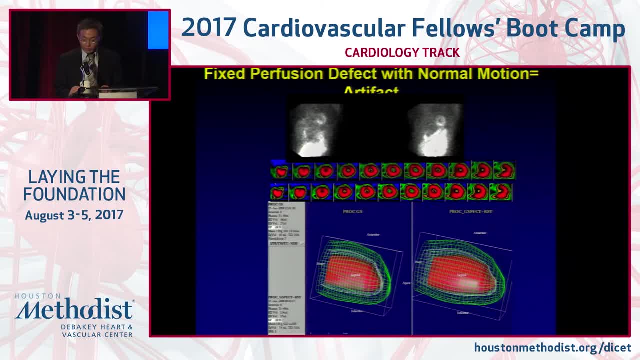 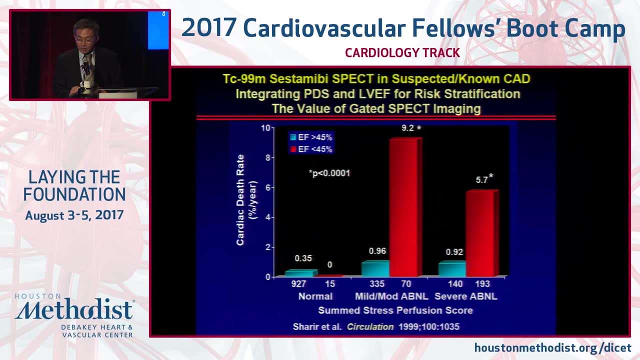 of disease, such as this case of women with fixed anterior defect. If you have the functional information showing normal wall motion, you can tell that this is artifact rather than true fixed defect or scar. Again, EF, in addition to profusion, add significant prognostic information for us to decide management. 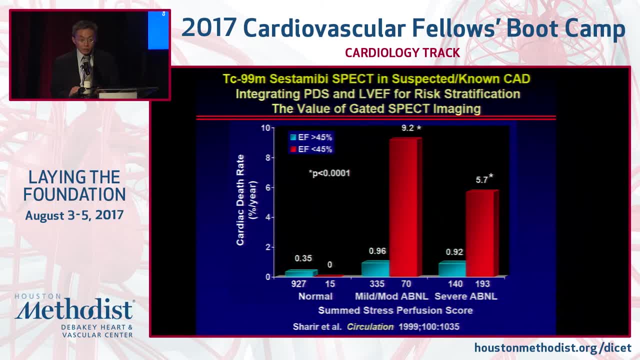 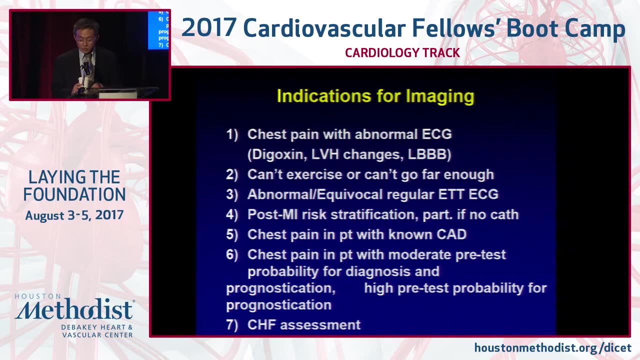 of the patient. So from the same study you can obtain profusion, EF and size. they all significant prognosis, significant predictor of prognosis. Okay, Thank you. What's the indication for imaging when you suspect somebody who had coronary disease? 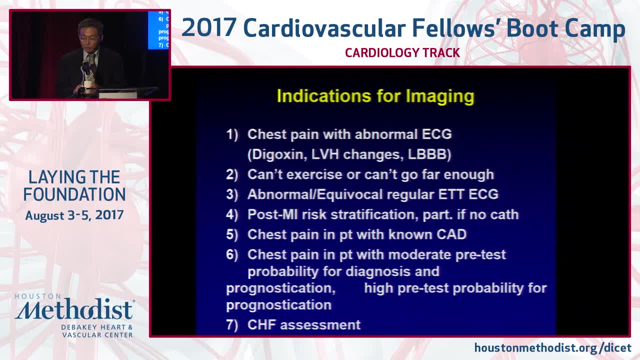 Obviously chest pain patient, especially with abnormal ECG ST changes due to LVH left bundle. patient cannot exercise or you have a patient, especially in women, with equivocal ECG Imaging. here I refer also to stress echo, obviously, but I think more and more the indication. 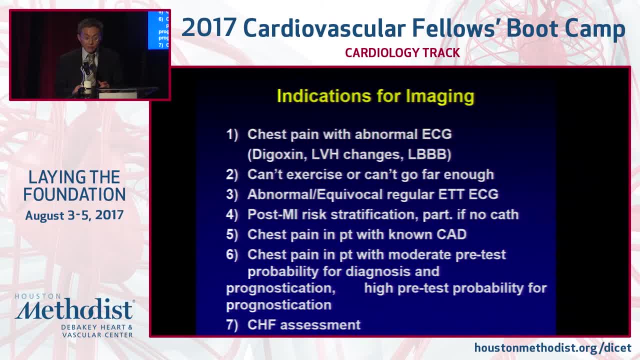 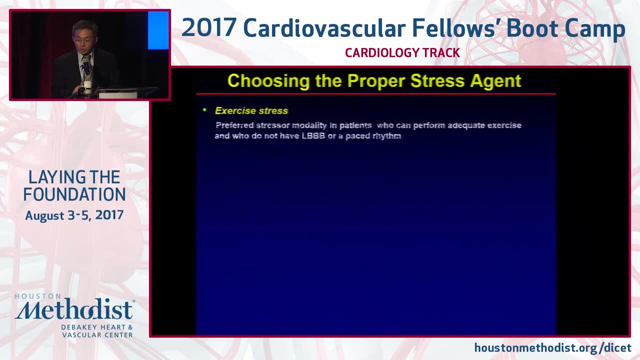 would be focused on patient with non-coronary disease. non-defect Okay In this. because of other imaging modality, who is available who could be probably better than stress imaging for determination of coronary disease? Okay, So what kind of stress test, as a fellow, you're going to order, right? 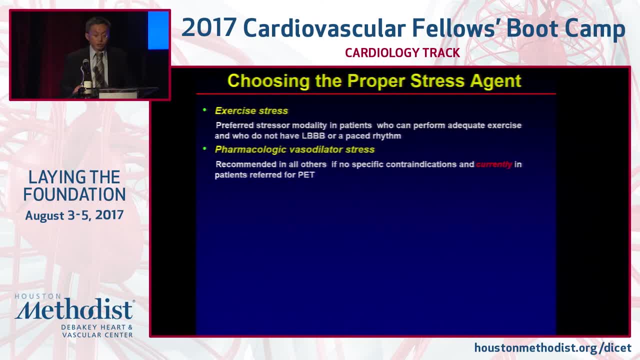 Exercise always prefer because you give you not only the profusion information, the functional information is also very important, especially for prediction of cardiac death or total death. Okay, But in the absence, in the presence of patient who cannot exercise, obviously, or have left. 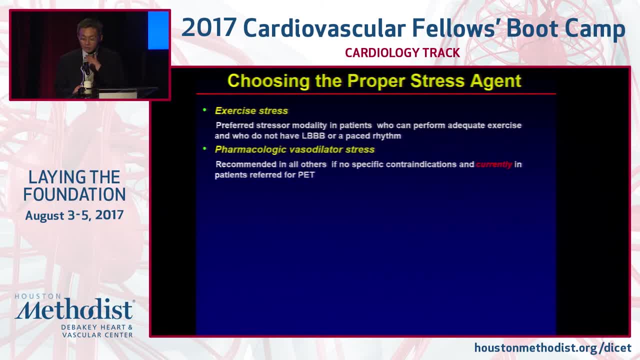 bundle, branch block or pace rhythm. here in Methodist Hospital a study was done here that vasodilator stress test using adenosine is much more accurate than exercise. Okay, So pharmacological vasodilator stress test recommended in those patient who cannot exercise. 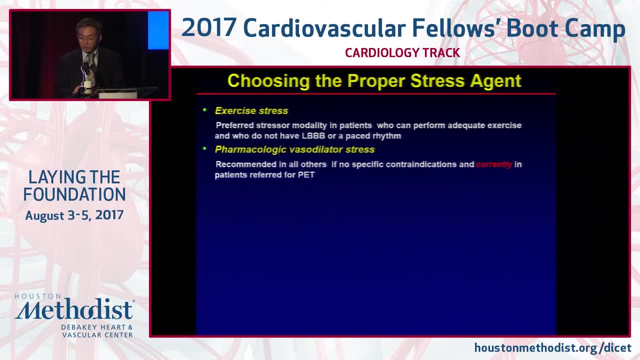 or have left bundle or LVH or pace rhythm Okay, And currently we. PET is preferred in large patient because of better photon energy, better suspect dobutamine. really we don't do that anymore. It's only very rare occasion with dobutamine, nuclear stress test. 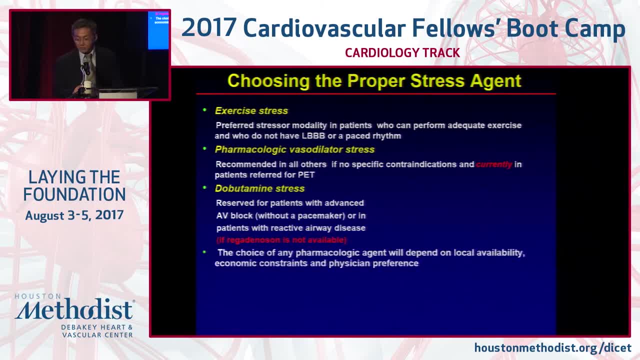 Okay. But the important thing, the choice of pharmacological agent depend, you know, you have dipyridamole, you have adenosine, you have Lexi scan- Okay, Or regadenosine, depending on the availability and depending on the cost. 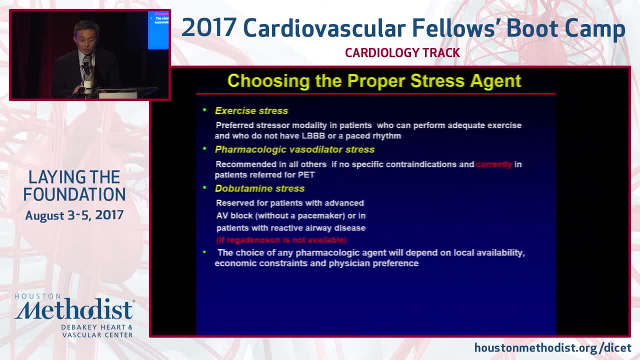 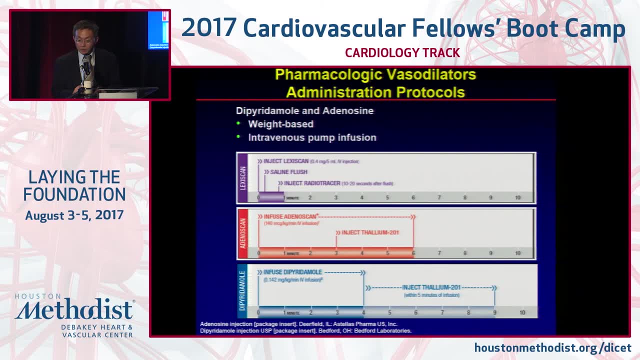 Here in the US, I think because of the ease of use, Lexi scan or regadenosine has becoming the preferred agent. So the protocol is very different. You can see the Lexi scan has become popular because, again, it's really easy. 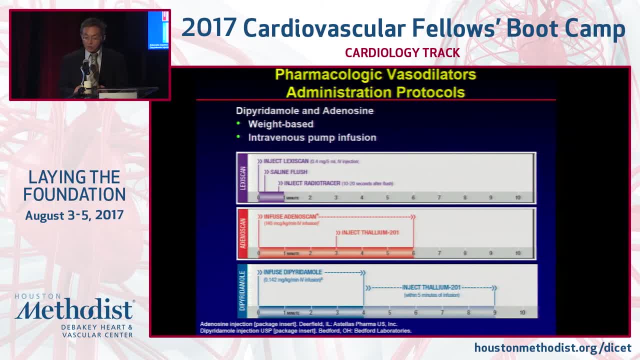 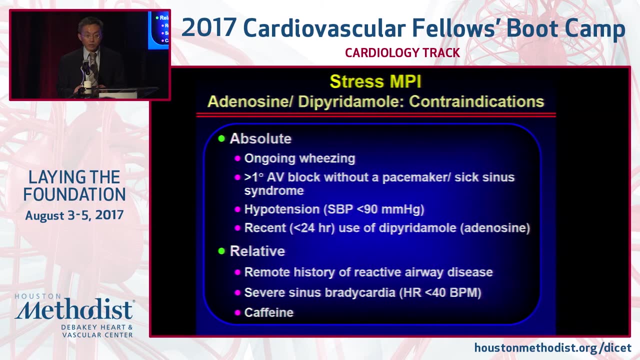 It's a bolus injection, So compared to dipyridamole and adenosine, which require infusion, Which is a lot more cumbersome, And the data showing pretty much adenosine and regadenosine has similar diagnostic accuracy and also it determine the size of defect. 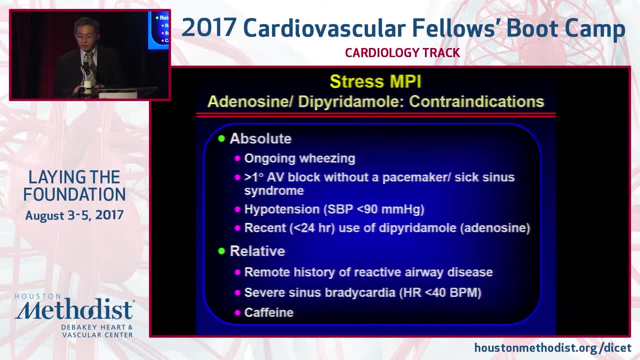 Okay For the fellows. obviously this is very important when you're in the lab to know the absolute contraindication for patient order. pharmacological stress test. Ongoing wheezing patient with history of asthma or COPD. If they're wheezing actively, do not give any adenosine or regadenosine. 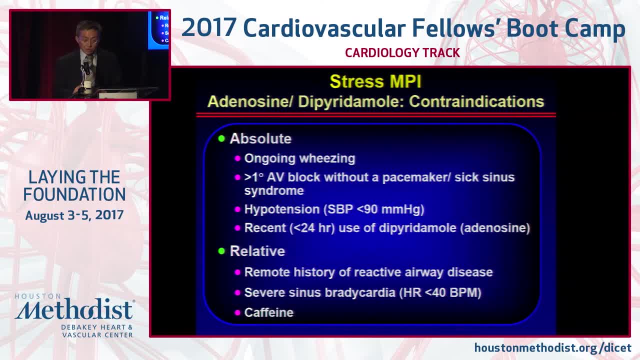 More than first degree AB block. First degree AB block is okay if you monitor closely. They have hypotension, especially in the presence of severe carotid stenosis. Okay, It's not a good idea. Or less than 24-hour history use of dipyridamole, especially in patient who is taking adenosine. 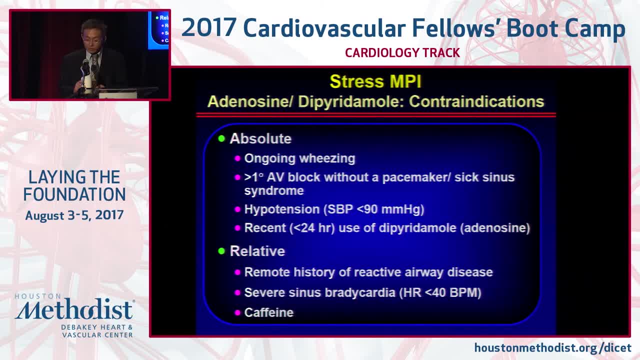 Patient who is taking dipyridamole and aspirin for stroke prevention Relative contraindication if they have history of reactive airway disease and not actively wheezing. regadenosine is a selective adenosine receptor blocker in the vascular bed. rather 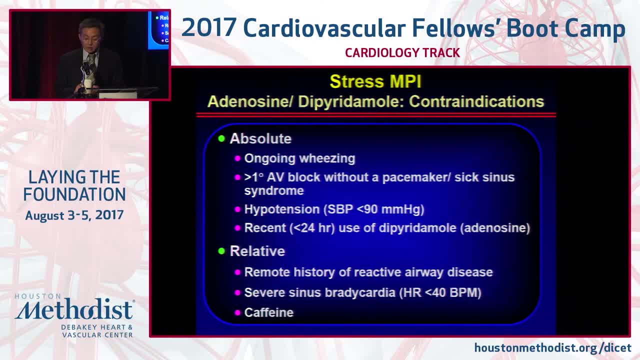 than bronchial or trees is very safer. Caffeine depending the coffee. how much amount Some studies showing it really doesn't affect the diagnostic accuracy. It might affect the defect size that you assess And obviously, patient with severe bradycardia conduction disease you try to shy away from. 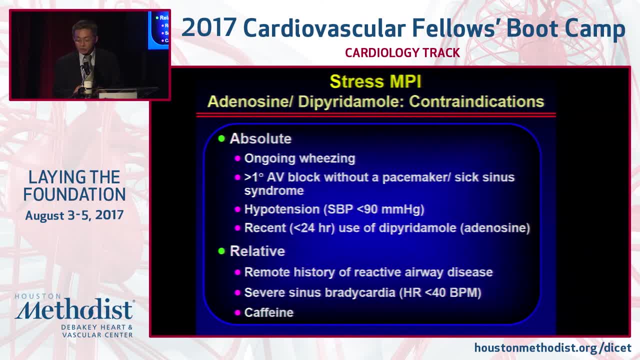 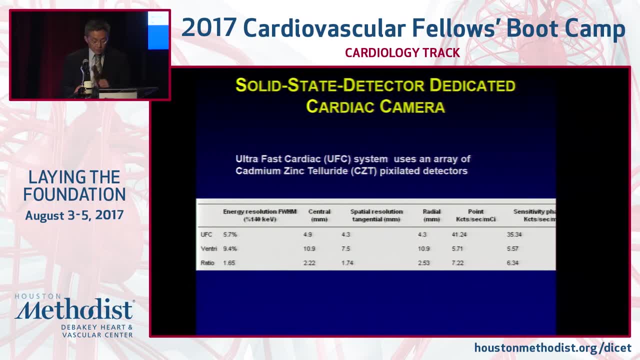 any agent like adenosine or regadenosine. This is a new. some of the new development: There's a new camera using solid state detector- ultrafast, because in the old scanner there's a traditional sodium iodine scanner. 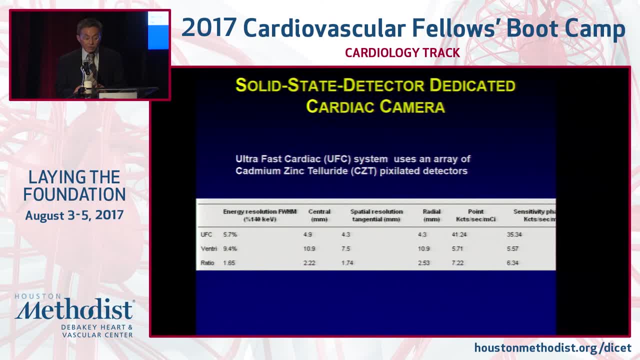 It takes you about 10,, 8 to 12 minutes, depending on the protocol, to acquire each set of picture. Okay, So for some patients, especially elderly patients who cannot stay still for a long period of time, it's a problem. 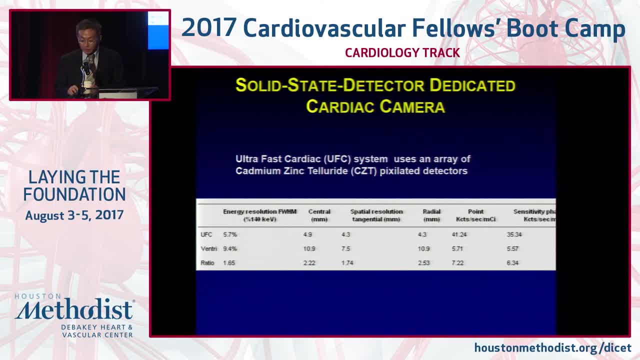 With this new camera which you can see there, compared to regular camera, so the UFC is called ultrafast system. Ventri is just a vendor's brand of regular camera. You can see The resolution. spatial resolution is much better: 4 millimeter versus 7.5 millimeter. 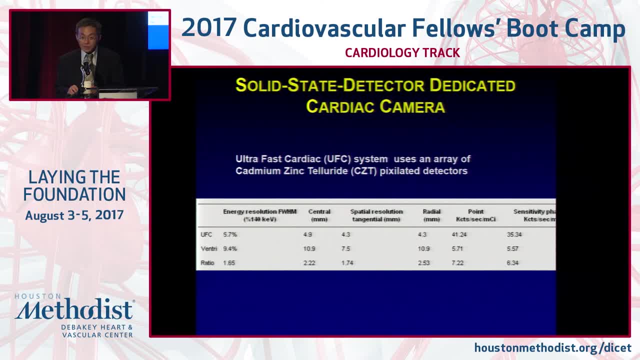 And sensitivity is about 6 times higher. So you can imagine, you can, since imaging image is determined by the number of photons. So you have more sensitive and more better spatial resolution. You can either image, you know, instead of 8 to 10 minutes, you can do 4 minutes imaging. 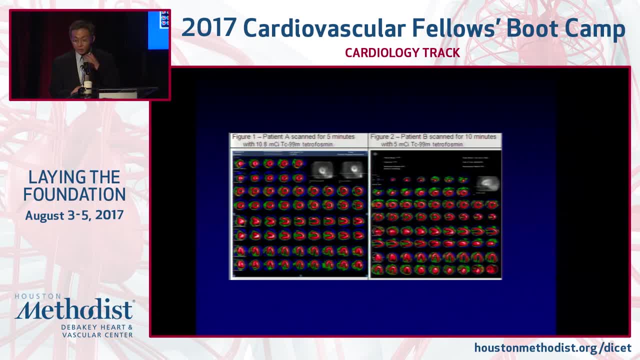 Or you can actually cut the doses in half And this is example of a patient, for instance, scan for 5 minutes with 5 minutes with 10 midi curie of tetrafosmin, which is a standard dosage. Okay, 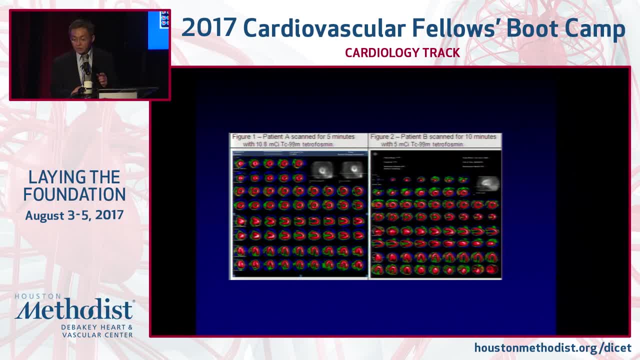 Or basically half of time. So you can do half time imaging in the left, Or you can do half dose imaging, Okay, So you're going to ultimately have similar amount of count compared to regular camera, So that allows you to do individualized imaging. 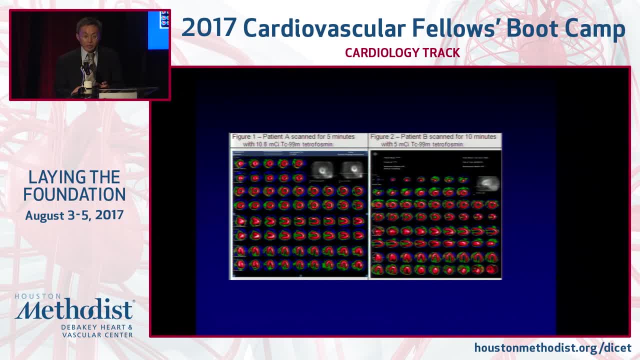 Let's say you have a young patient, You don't want to give too much radiation. You can imaging them with 10 minutes. Okay, With half of the doses of radioisotope In the elderly patient who cannot stay still for a long period of time, you can give them. 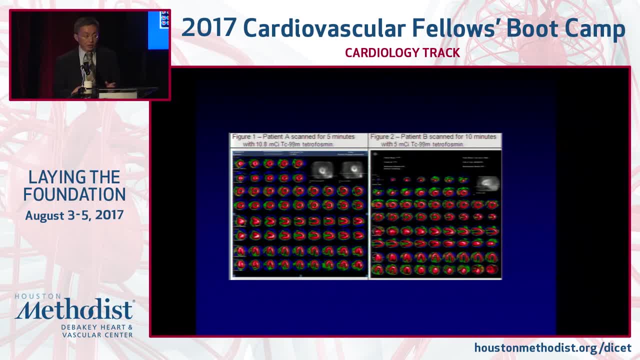 regular dosage of radioisotope and imaging half of the time. Okay. So this new development allows you to customize the problem, The protocol, Okay. So that's all I have to say about nuclear. A really quick introduction.